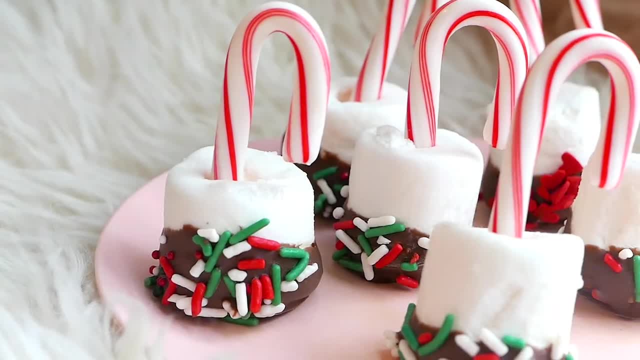 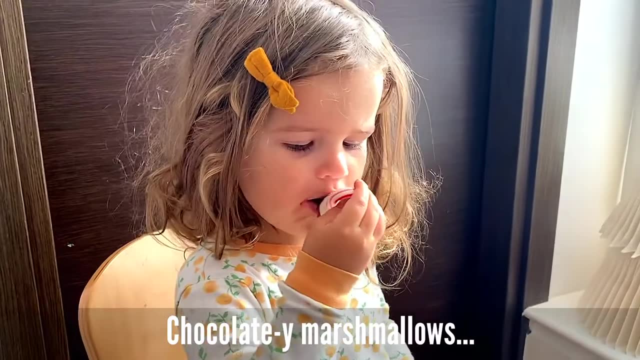 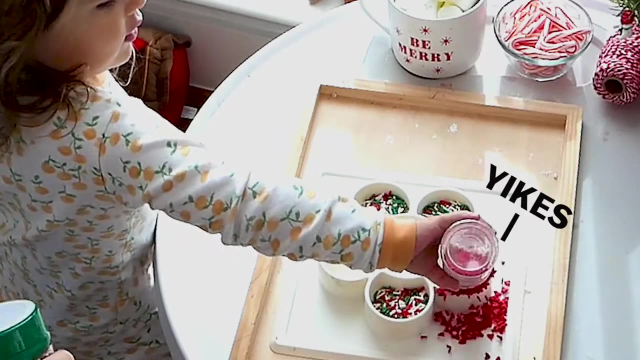 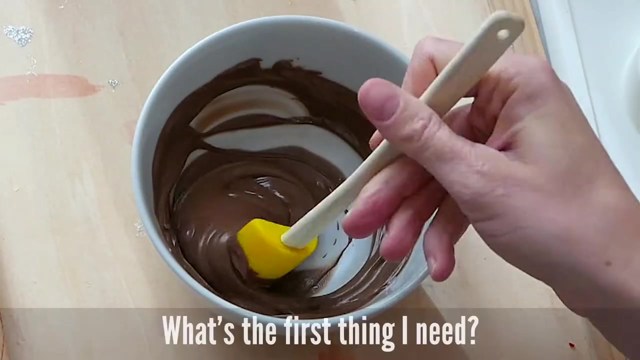 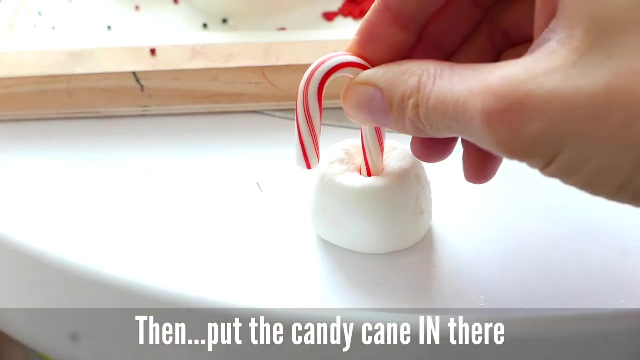 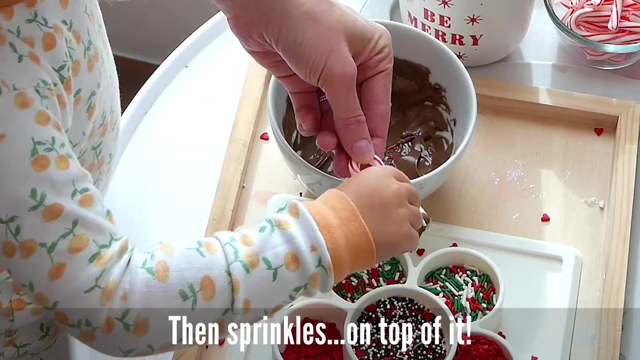 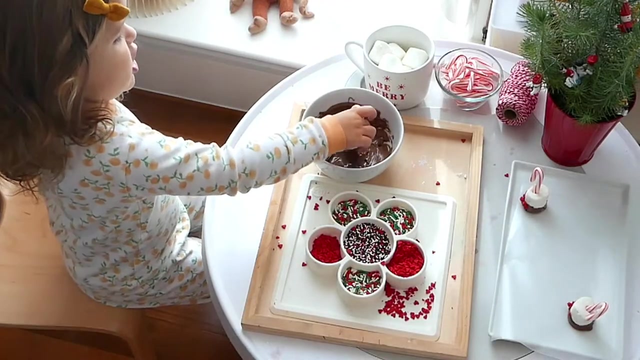 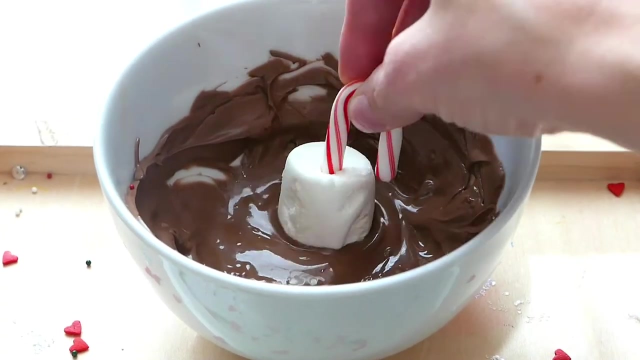 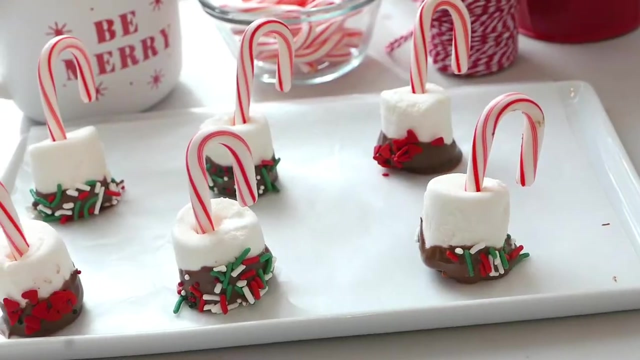 What's the first thing I need? I need a smile, then put a chat in the chat and then use those to put into a topic. This is a topic. Hi, my name is. Hi, my name is. Hi, my name is. 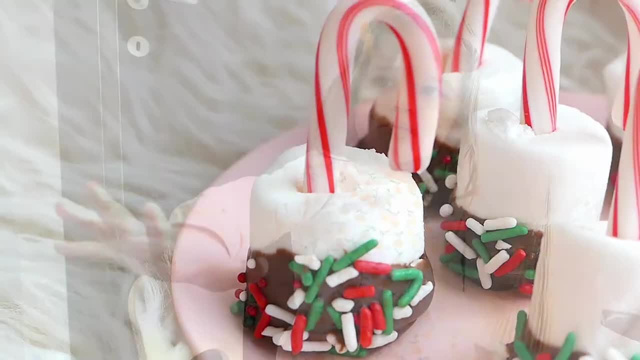 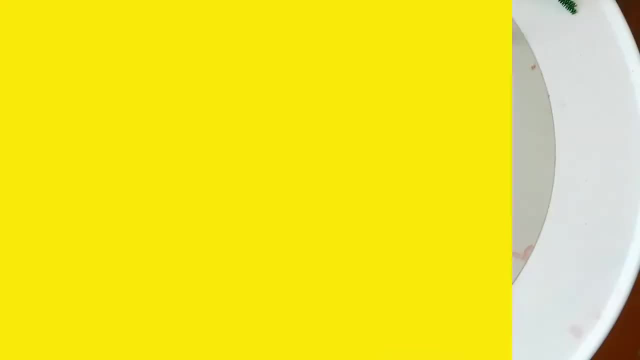 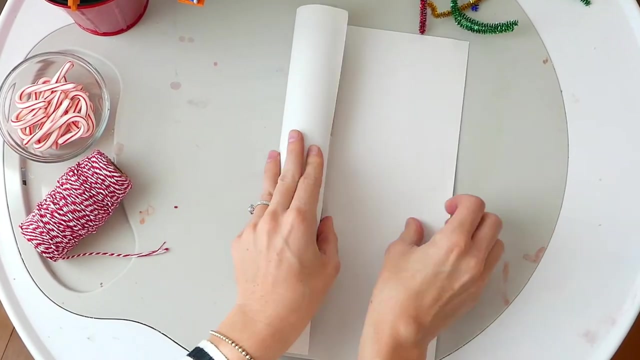 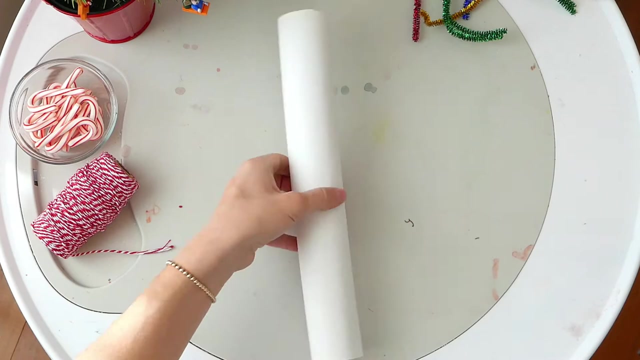 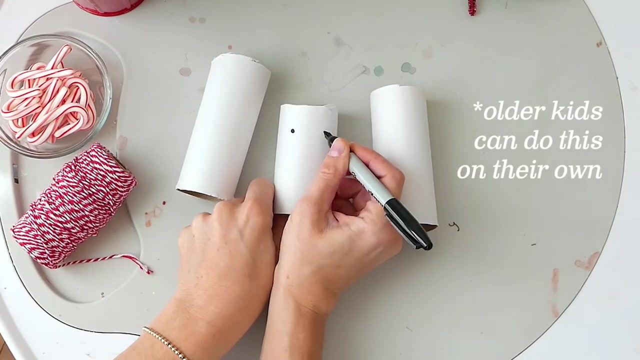 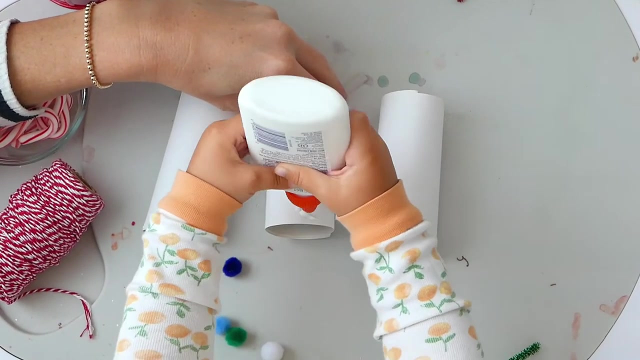 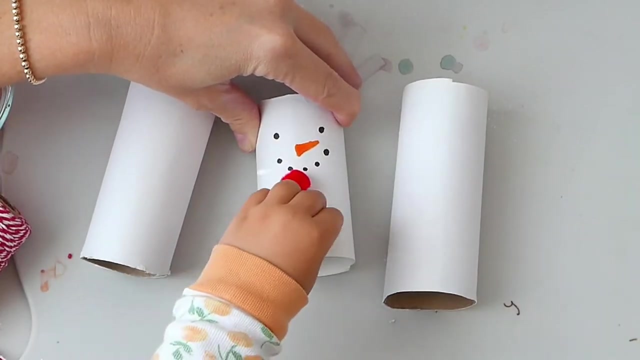 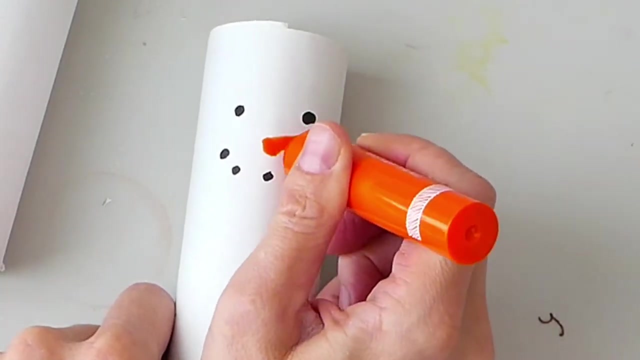 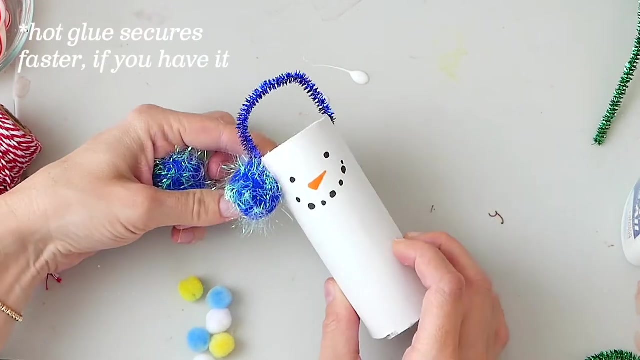 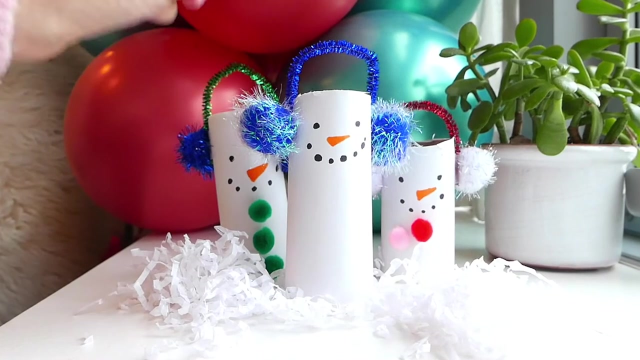 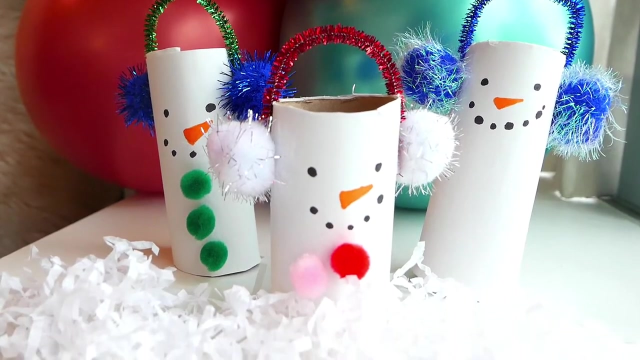 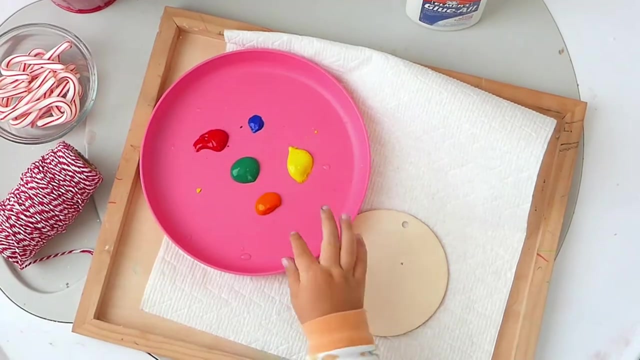 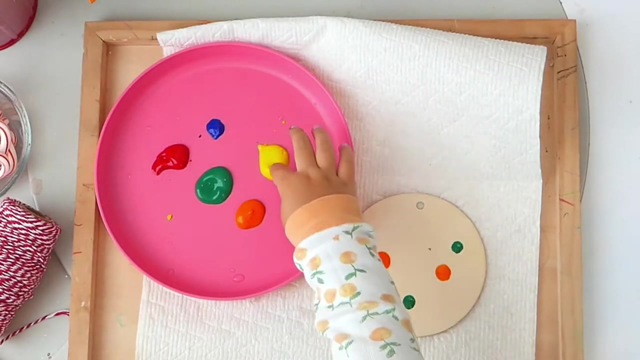 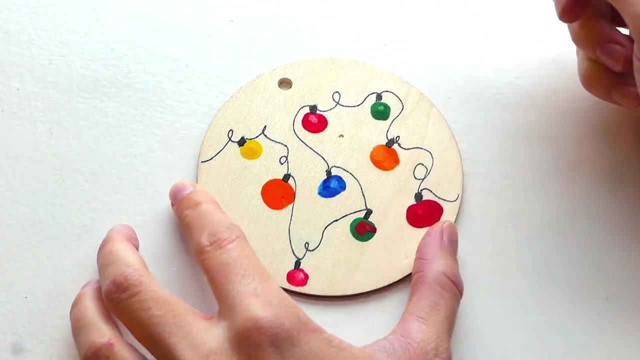 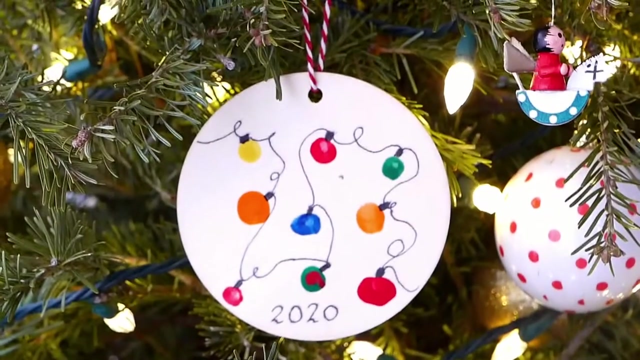 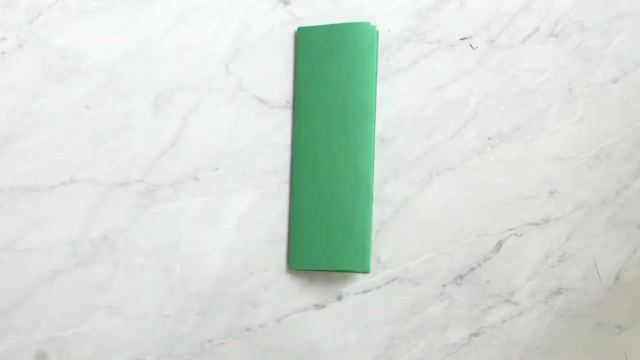 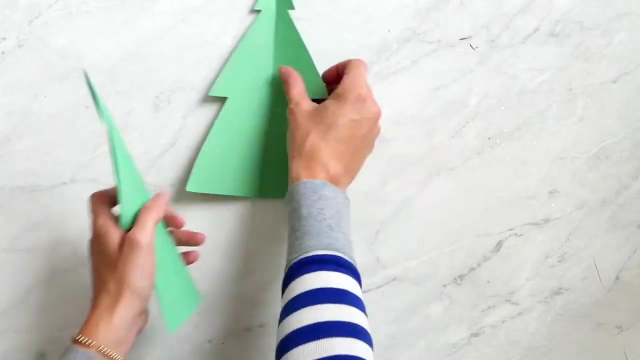 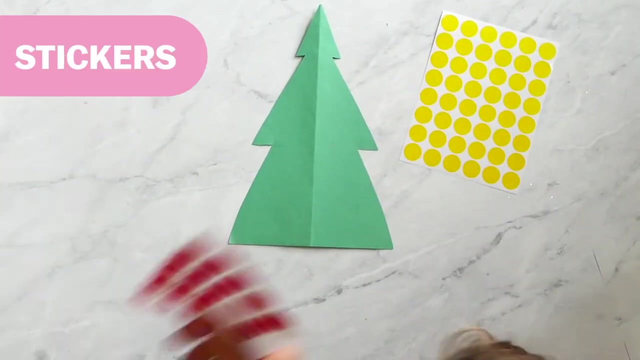 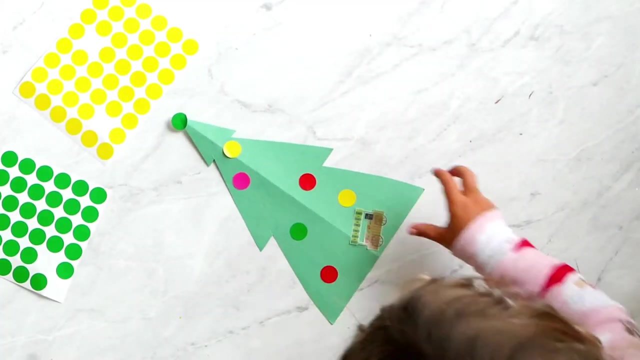 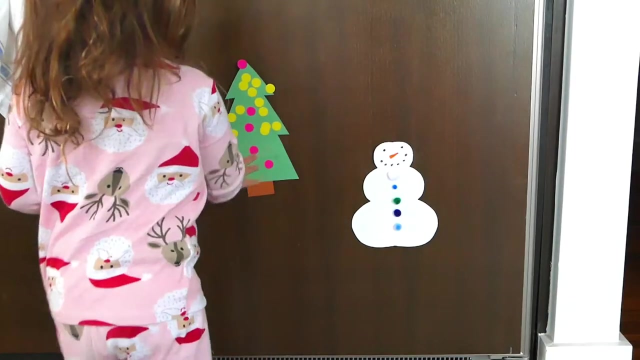 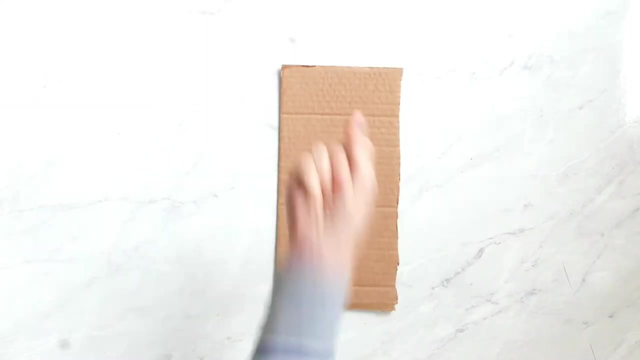 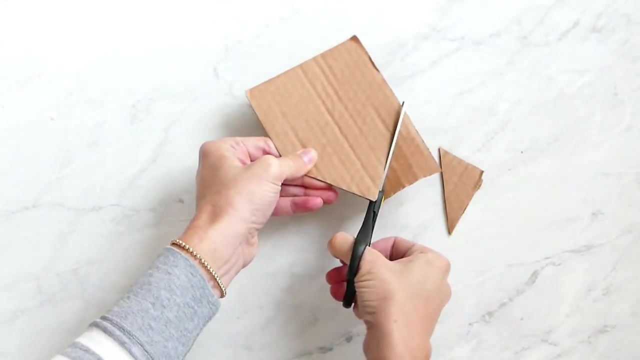 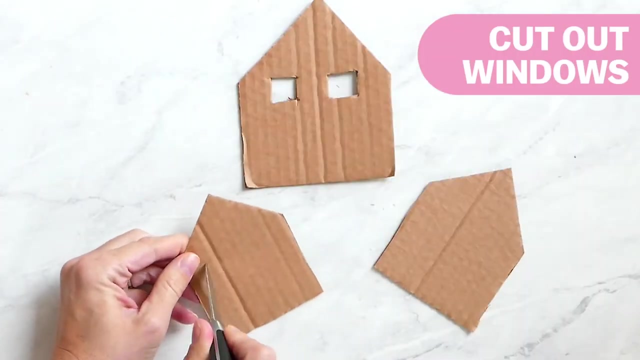 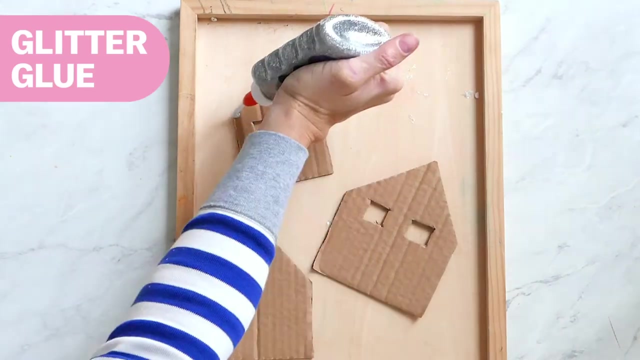 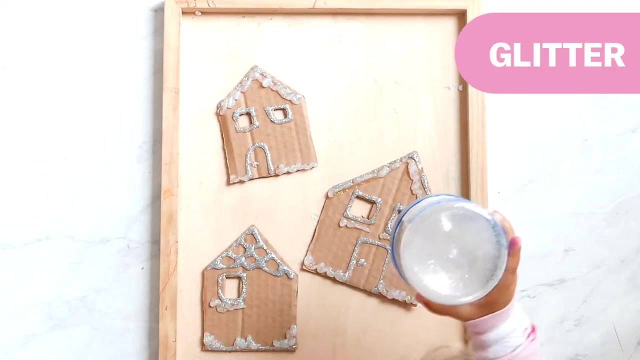 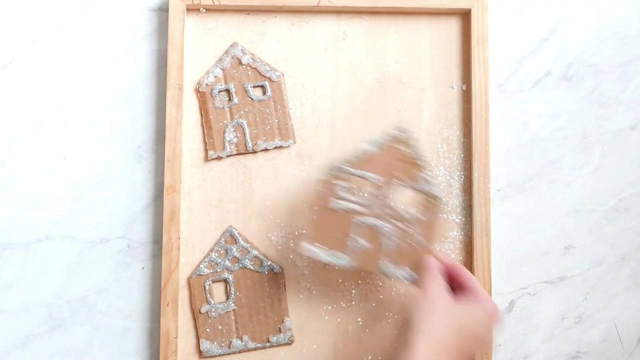 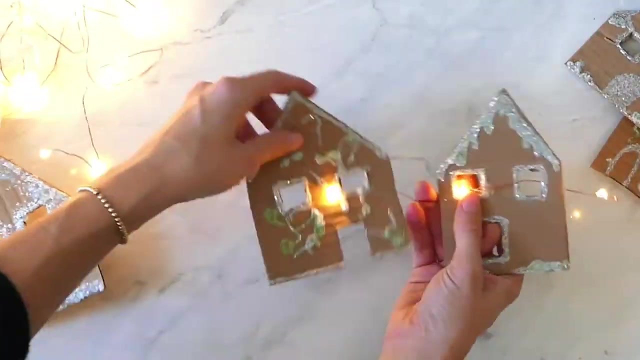 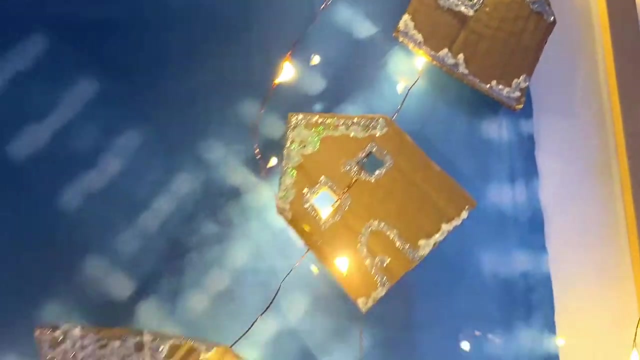 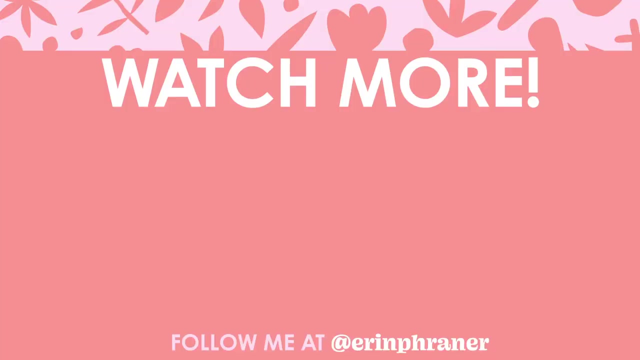 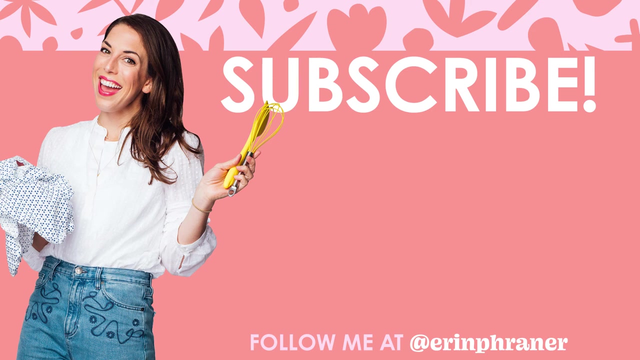